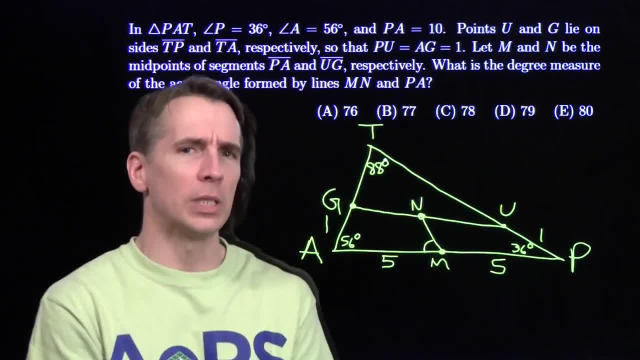 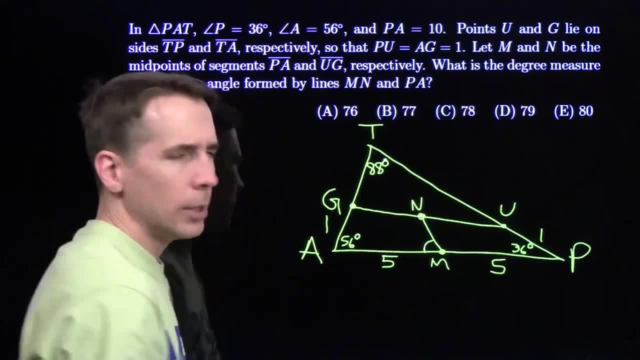 in terms of that variable. before we do anything, We want to think a little strategically, Think about what is it we're probably going to have to use. What information have they given us? here We see these two equal lengths and we think, well, that's got to be important. 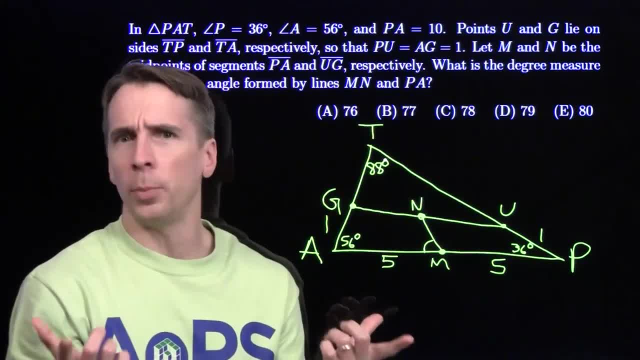 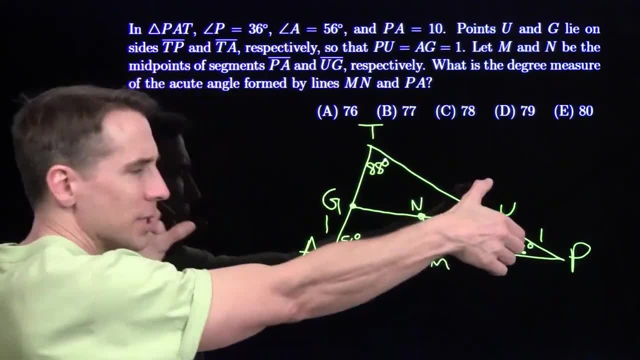 somehow We've got to be able to use these equal lengths. Now, how do equal lengths help us with angle-chasing? Well, they might give us a parallelogram, but clearly these two are not parallel. They're not opposite sides of a parallelogram. The other place we see. 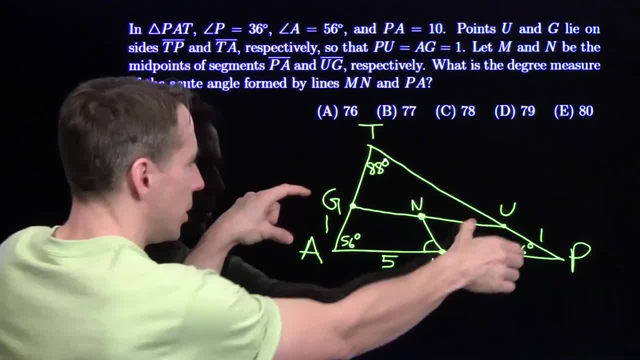 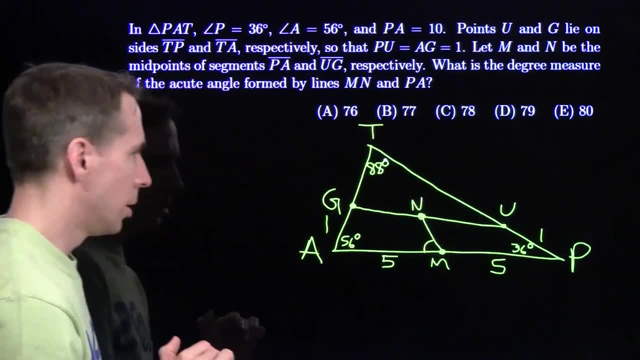 equal sides is in isosceles triangles. These aren't even connected. If I could somehow get these two together, build an isosceles triangle, that would help me with some angle-chasing. I don't see it right away. The other thing: 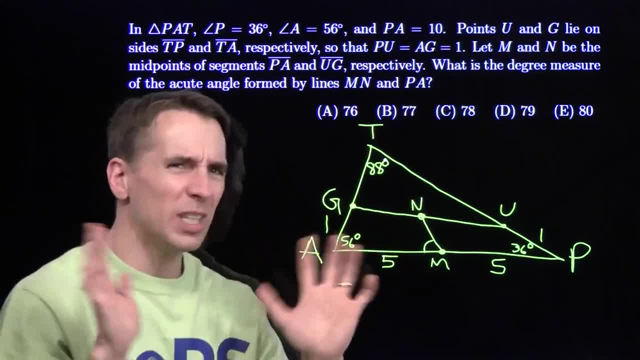 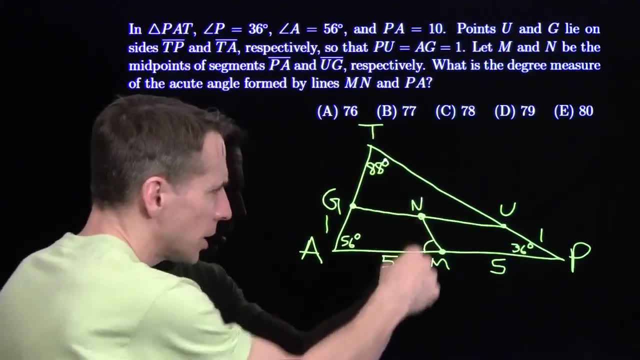 I see is I see these midpoints. They told us something about midpoints. We haven't used any of that information we have about these midpoints, And I start thinking midpoints and angles. How do midpoints help us with angles, especially connected midpoints- Connected- 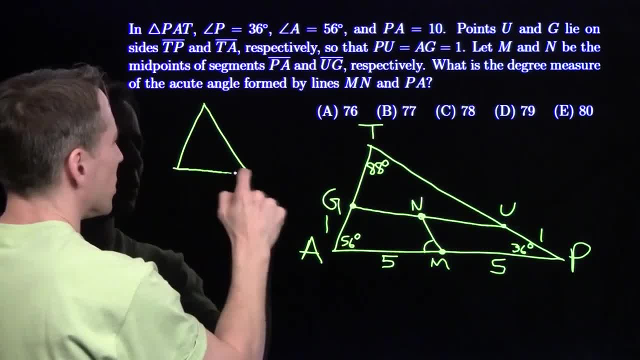 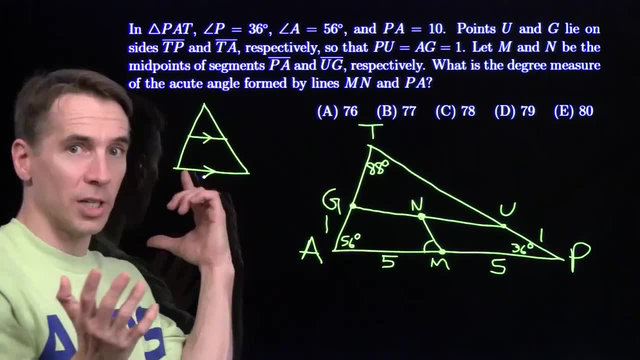 midpoints and angles. I start thinking about connecting the midpoints to the sides of a triangle, And when you do that You form parallel lines and you've got some angle-chasing there. Clearly, we can't do that here yet either. So I've got these two things rattling around in my head. I've got these. 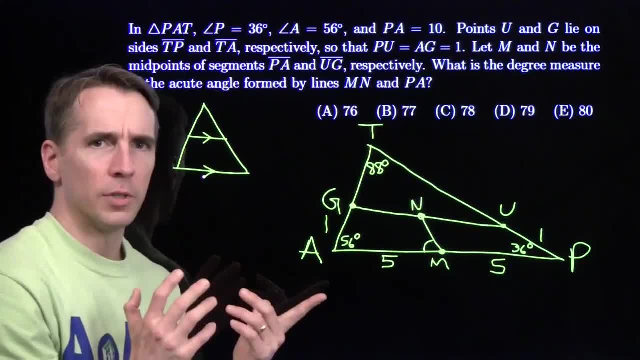 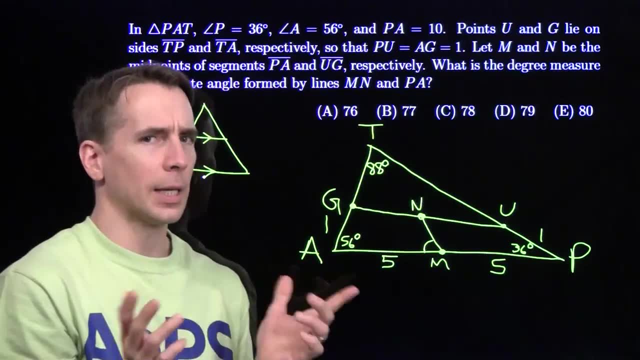 ones here, and I've got this diagram here- connected midpoints of a triangle. All right, see if we can use that as inspiration. What I'm going to do first here, instead of throwing in variables, I'm going to look for points to connect in my diagram to help me with some. 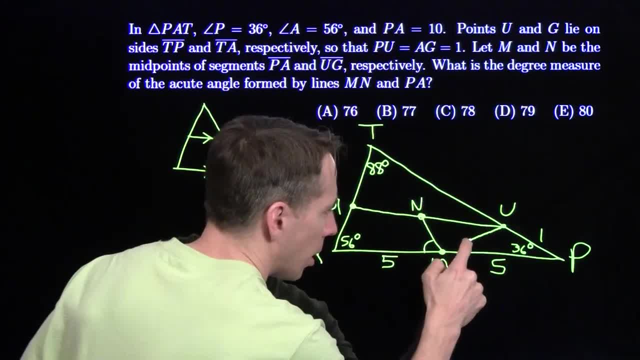 angle-chasing And a natural choice here. I'm going to go like this: I'm going to connect u to m. The first thing I'm doing here is: I'm starting to build this triangle. I'm going to connect u to m. I'm going to connect u to m, And the first thing I'm doing here is I'm starting. 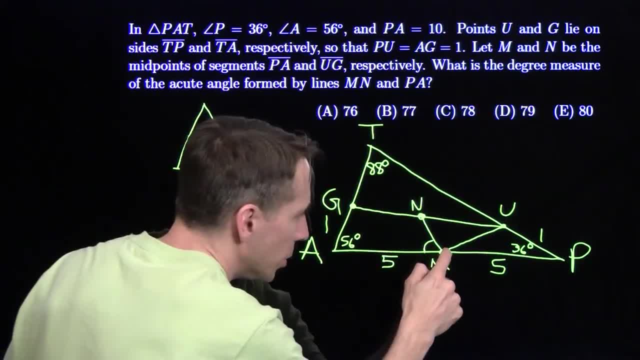 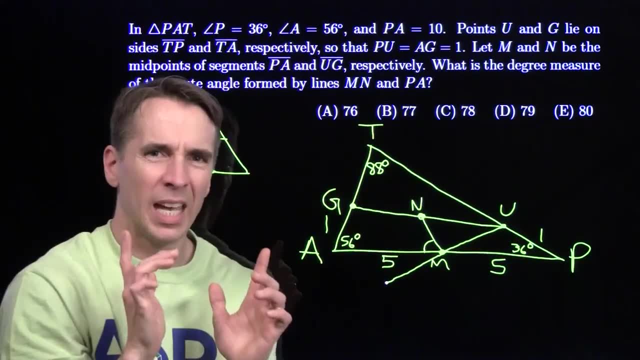 to build this diagram here. I'm going to continue it on, And the other thing I'm doing here, as I continue this on, is what I really want to do. I want to bring this one over here. I want to connect this one to this one, build an isosceles triangle. So I'm going 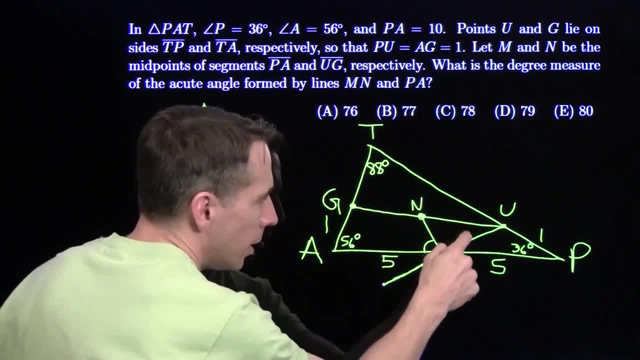 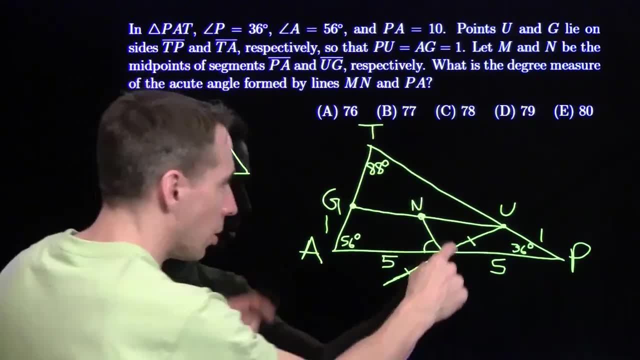 to keep going. I'm going to keep bringing this out here. the same distance I have here. So this equals this And we already have this equal to this and these two angles are equal. So when I connect these, I have this triangle right here is congruent to this triangle over.